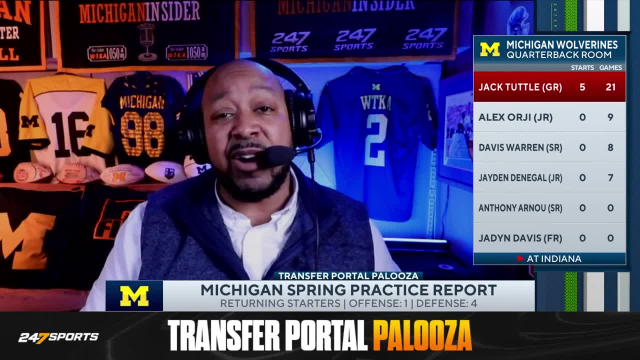 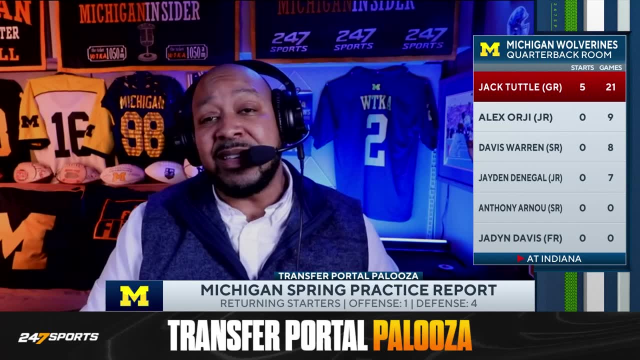 able to maintain the culture, You're able to maintain the pieces around the quarterback that will allow him to be successful, but maybe in a different kind of way, And it looks like Alex Orji right now. I think it's very much a competition. You got Alex Orji in the mix. 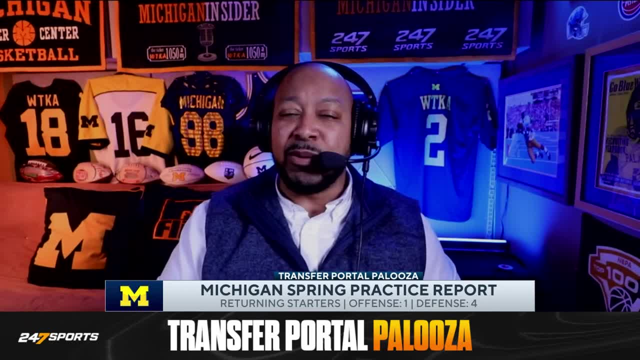 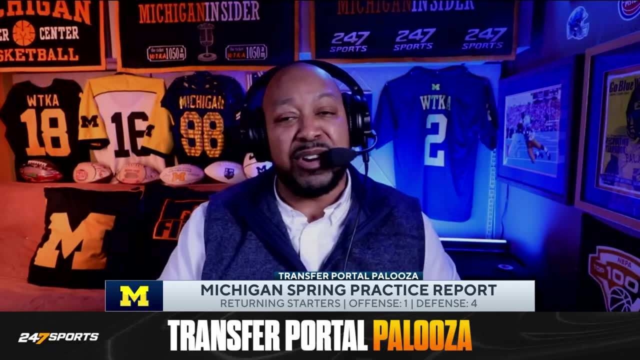 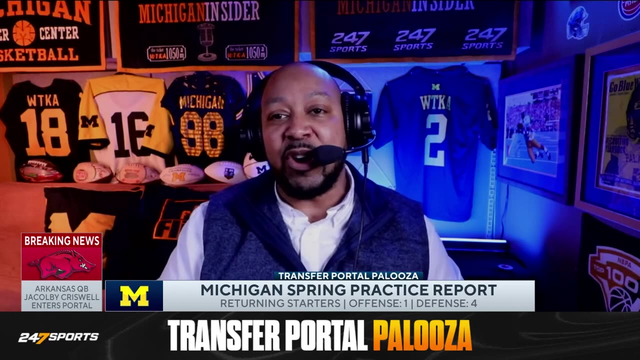 as a dual-threat quarterback, a guy who cerebrally, I think is very similar to JJ but is not the same skill set. I mean, you're talking about a guy who is 235, a legit four or five guy is going to be able to get you some of that production on the ground. 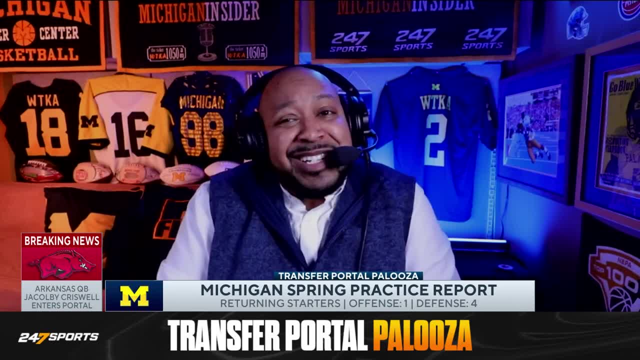 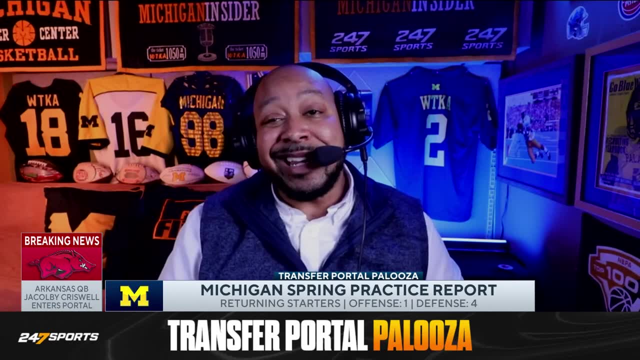 that JJ was capable of, but you didn't emphasize it as much because JJ was 200 pounds. right, He was definitely more of a pocket guy than an Alex Orji is going to be, But in this scheme with an 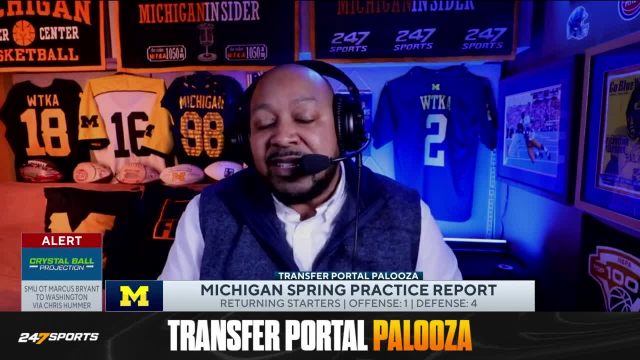 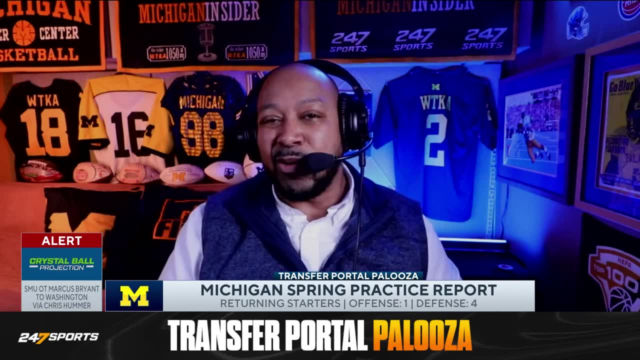 offensive line that you're going to replace. you got to remember they're going to be replacing their entire offensive line. There's probably going to be a need for a guy with some more movement back there, which is why Alex Orji, I think. 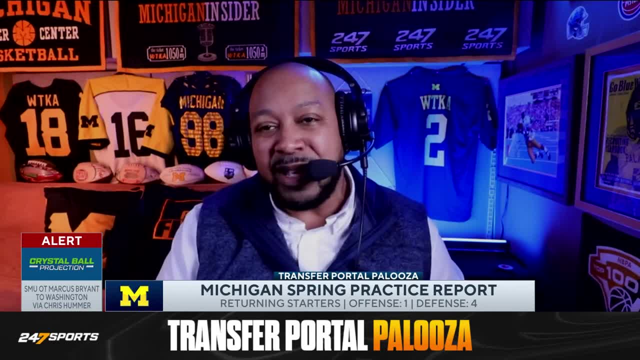 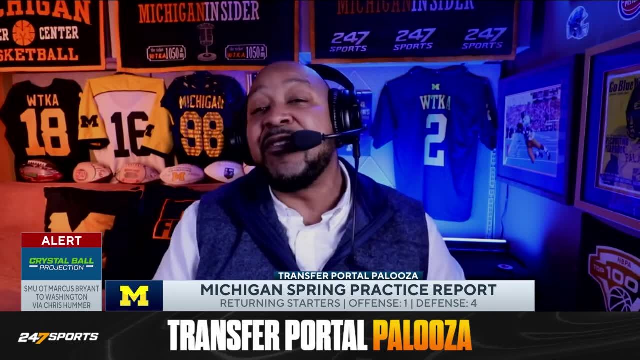 is beating the pack at this point. That's not to say that he can't do a lot of the throw things they're going to do. I think you're going to see aspects of the offense have a different emphasis. So they had QB counter in there, a lot of the QB run stuff in there with JJ. He didn't call it as. 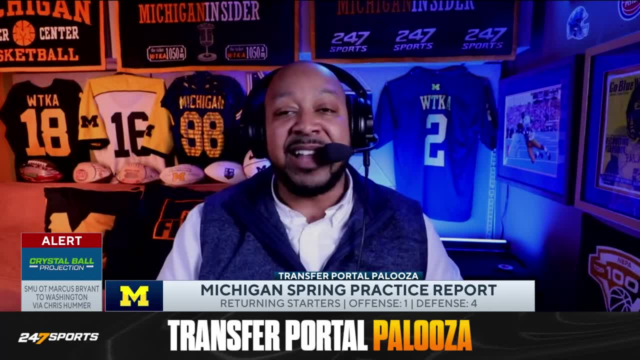 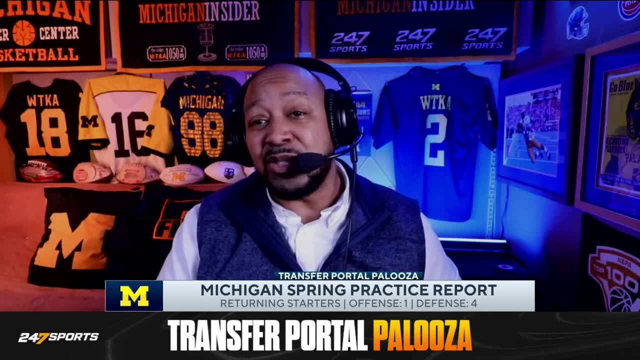 much You're going to call it more with Alex Orji. if he's the guy, I think the reprogressions will be different. JJ had a lot of whole field reads in his arsenal. This one, if it's Alex Orji. 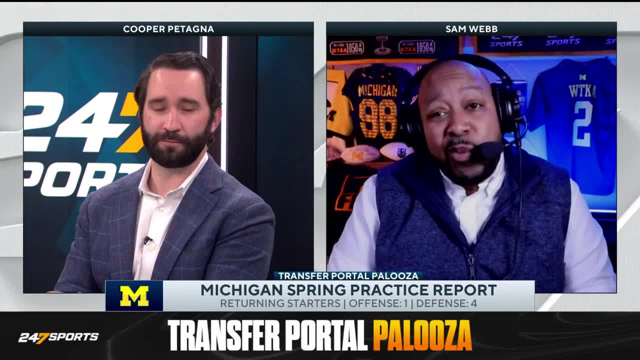 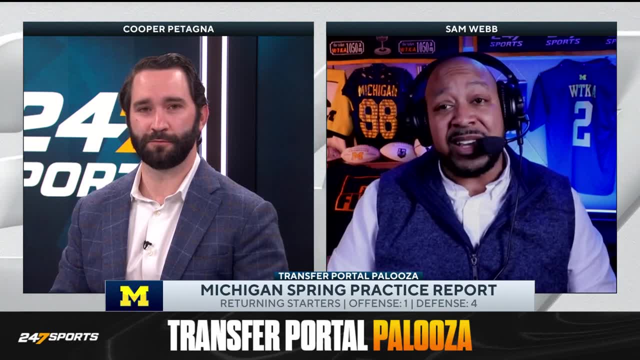 probably one, two then run, But he has to win it. He has to hold off of Jaden Denigal. He has to hold off of a guy like Jack Tuttle who has started games at the college football level and is nursing some injuries. 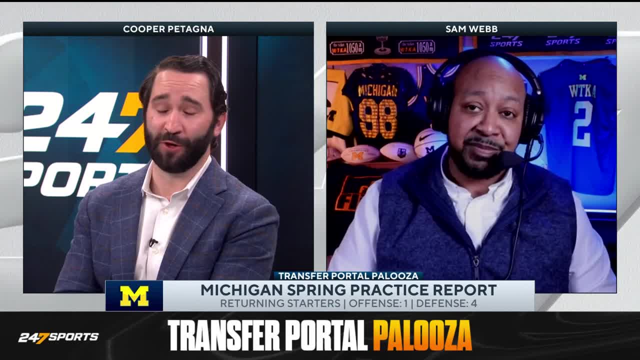 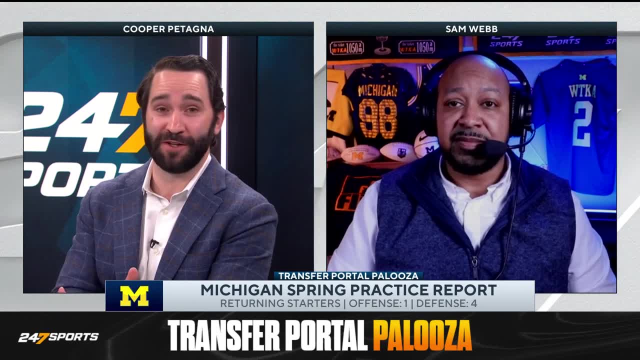 right now but will be in the mix when the ball rolls around. It's going to be a really interesting room. I mean, you mentioned Alex Orji going to be a different type of quarterback than what we saw from JJ McCarthy, And you also mentioned the. 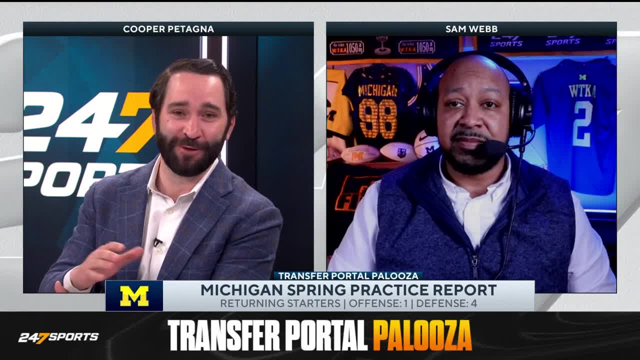 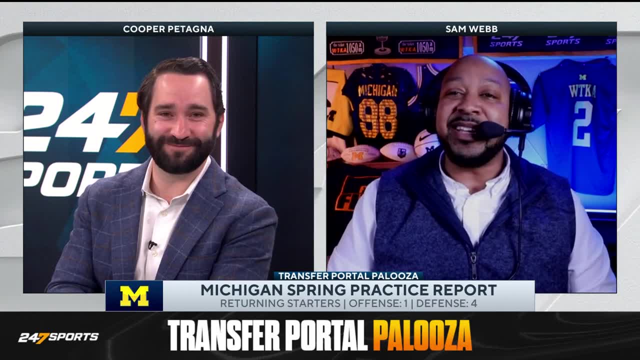 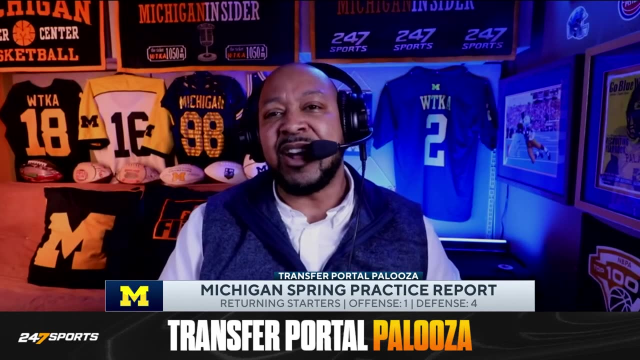 other caveat of this is that Michigan's got to replace that really, really talented offensive line. So, Sam, I ask you, how are you going to deal with that? How in the heck do they do that? Yeah, so it's different in that, while you lost starting, a lot of guys with a lot of start. 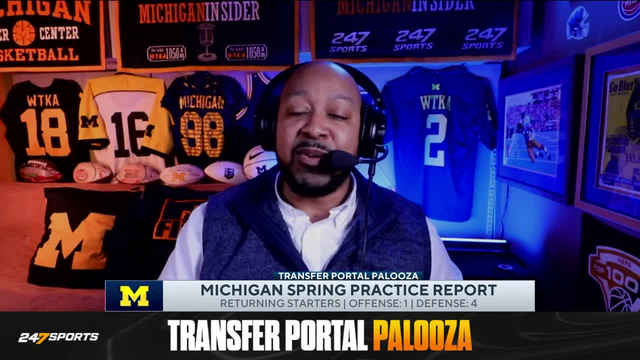 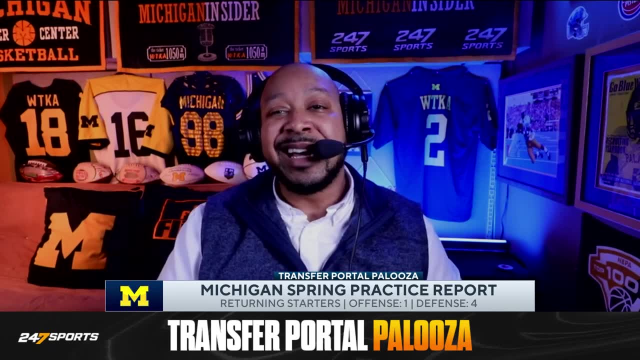 you're returning guys who have played a lot of football over the course of the last few years. Now, Miles Hinton started a lot of games at Stanford. He came in immediately, won a starting job here at Michigan, got injured and wasn't able to get that job back. That's a guy who 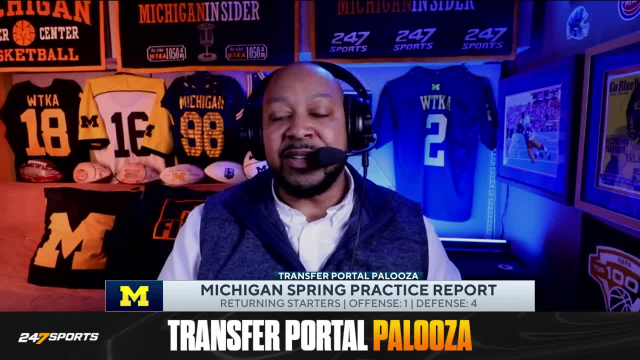 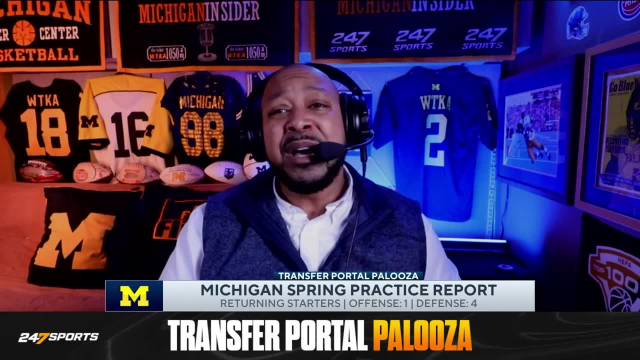 is a proven starter. After that, though, you're talking about a guy in Josh Preeb who comes over from Northwestern. He started a lot of games in Northwestern. He's still learning his system, But you get some experience at least playing college football. You look at Greg. 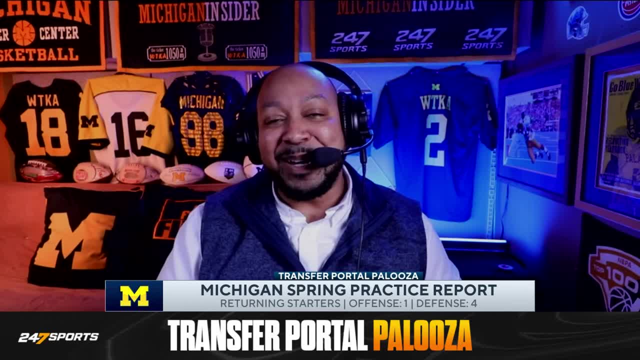 Crippen and he's a guy that's been in the circumstance that I heard. you know you guys saw Carl was talking about. If you haven't played one or two years you probably get lost in the shuffle. That's kind of Greg Crippen. I mean a couple of years ago you bring in Olu Olu. 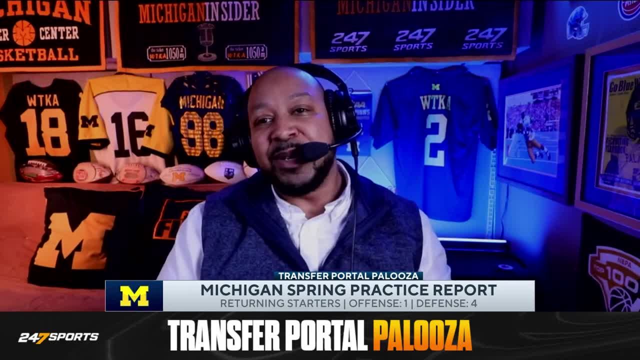 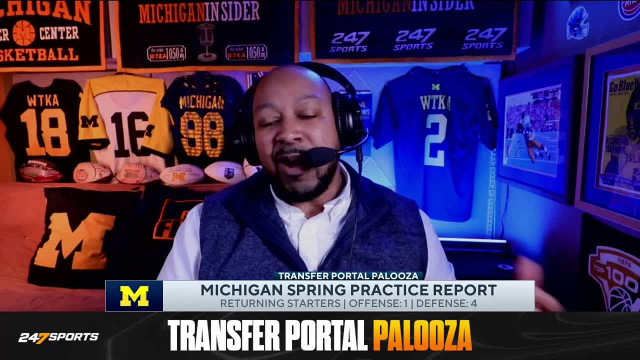 and Timmy from Virginia. He comes in and wins the Remington Award. Then last year you get Drake Nugent from Stanford. He comes in. He starts every game. Greg Crippen probably starts on a lot of teams across college football. He got some snaps at Michigan. 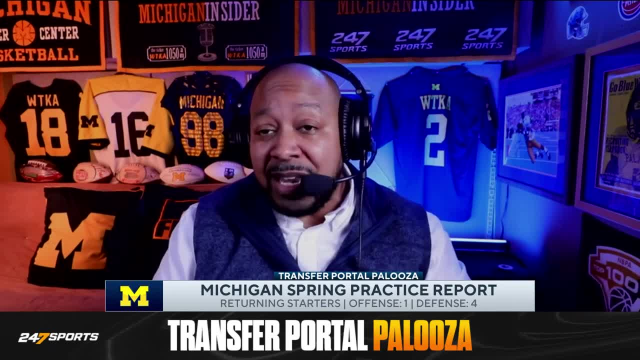 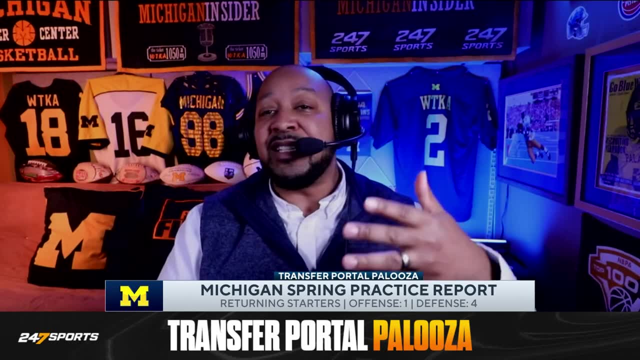 wasn't able to start. That's a guy that they were able to develop, though, and I think he's going to be ready to go. And then Giovanni Ohati at the other guard spot. He's played a lot of football. He's filled in for guys who were injured, whether it be Trevor Keegan, who had 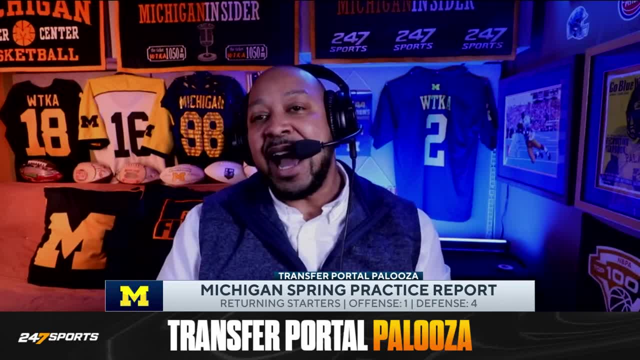 some injuries, or Zach Zinner at times. So he was a highly rated guy who's played some football. hasn't started. I think they feel comfortable with those four. The real battle is at the other tackle spot, where there's some inexperience. Probably it'll be between Alex Gentry, who was 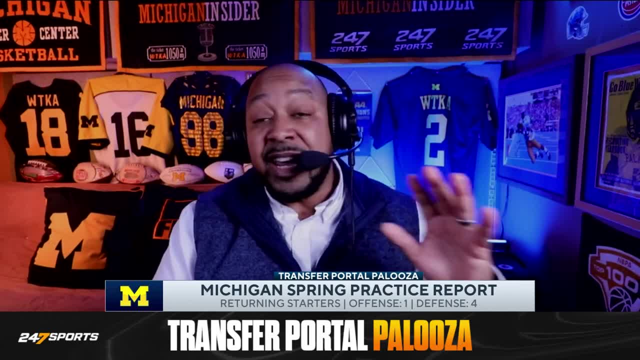 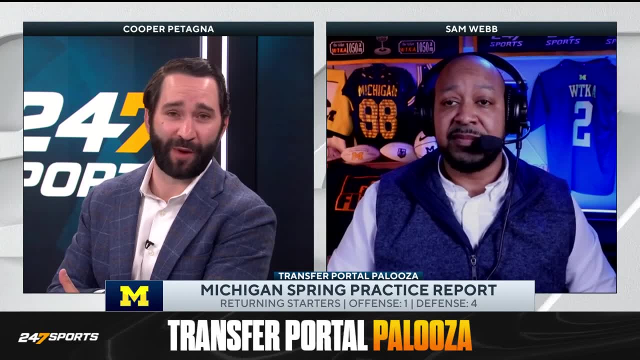 a top 247 guy and Jeff Percy, And then I think Michigan will go looking in the portal to help fortify the competition at that position. Sam, there's no question marks on the defensive line, especially when you talk about the Bash brothers and Mason Graham and Kenneth Grant. 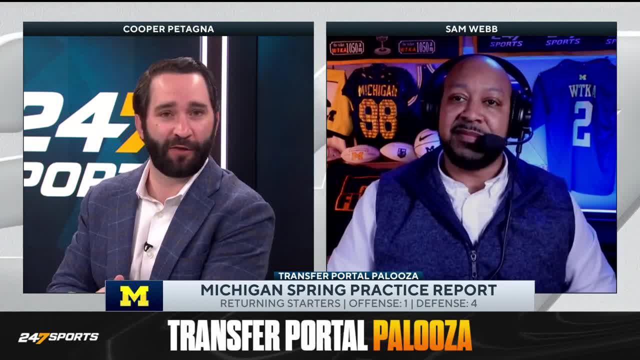 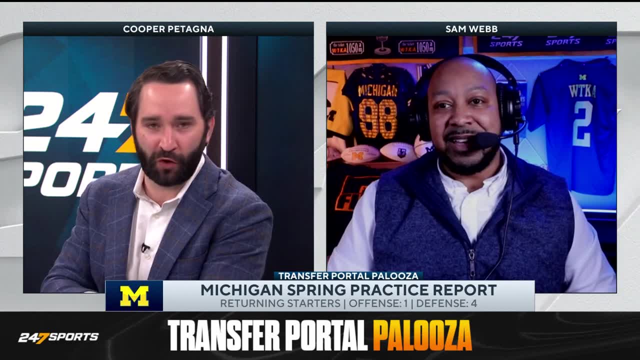 Those two are the best at their position in the country and I don't think a lot of people are interested in them. How good do those two guys have to be for Michigan to return not only to a college football playoff appearance but to repeat as national champions? 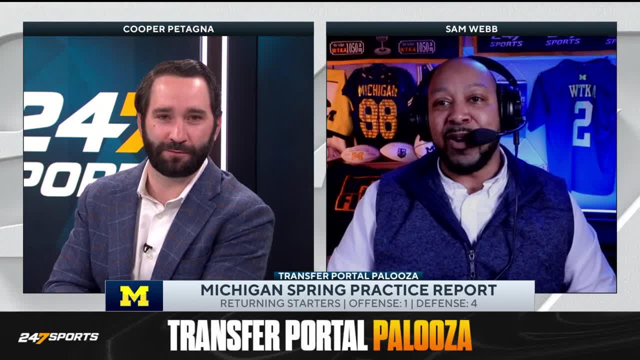 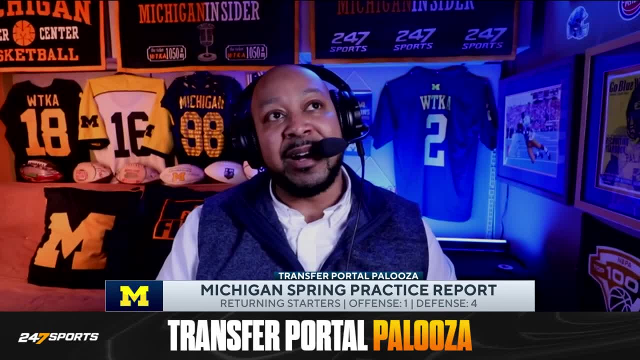 Yeah man, They are grown men. I was about to cuss on air. Those are grown men playing in a college football game. Mason Graham. I remember going to watch him in high school. You marveled at how a guy like that could be overlooked by all the local USC, UCLA, Washington. He was committed to boys. 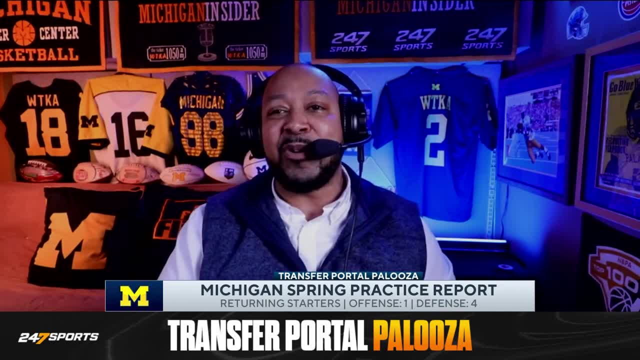 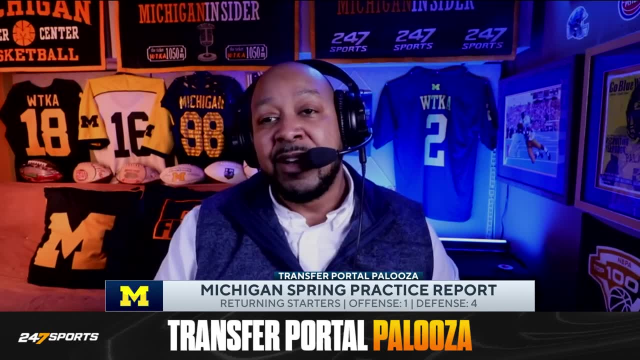 state initially, when my man, Courtney Morgan, shout out to Big Court, who is the GM down in Alabama now recognized this is a guy that Michigan should be on And they pulled him from Boise State and held on to him And what you saw? what I saw when I went to watch him in high 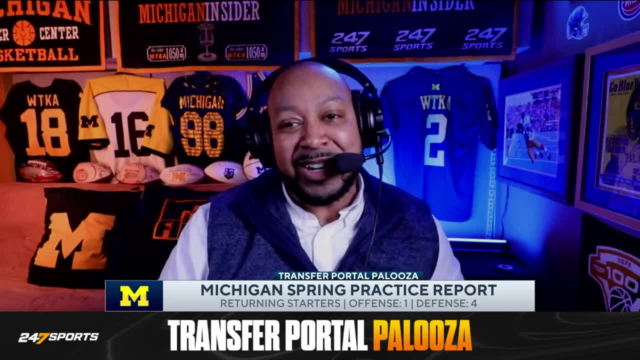 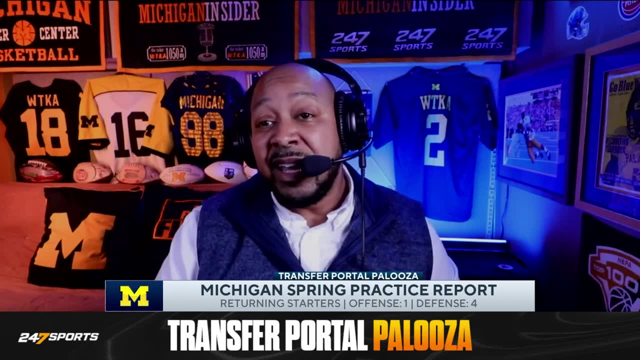 school was this dude. he played every snap along the defensive line, every snap along the offensive line and he played special teams. He had a motor like I had never seen and it translated to him starting and starting as a true freshman at DC. 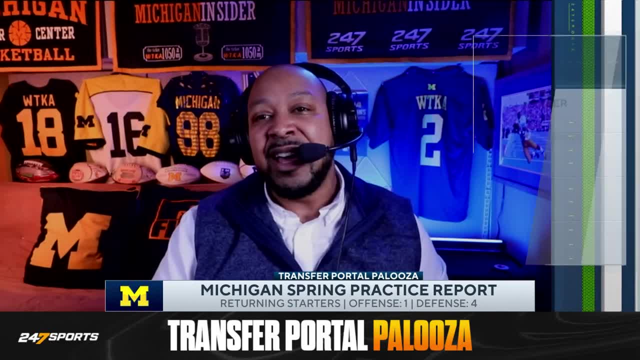 I mean he was a great defensive tackle. It was a package, but still he was a starter. You don't see that for interior lineman. He just knew he was going to be a dude. Took a little bit longer for KG to break the starting. 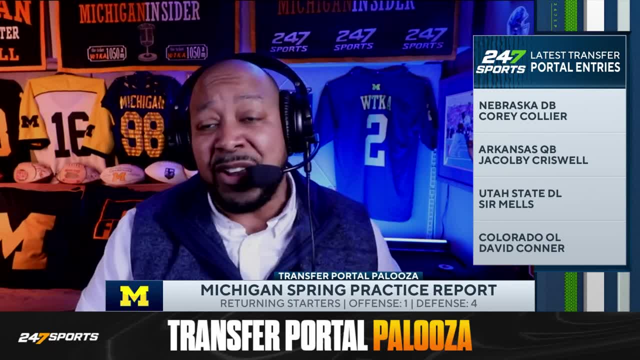 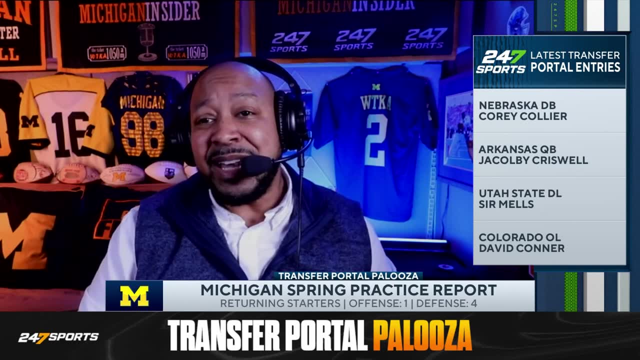 line. but once he did you saw that he was really really special. You saw him hog down a Penn State running back in the game last year from behind. Just next level talent. They're going to be, I think, on a higher level. 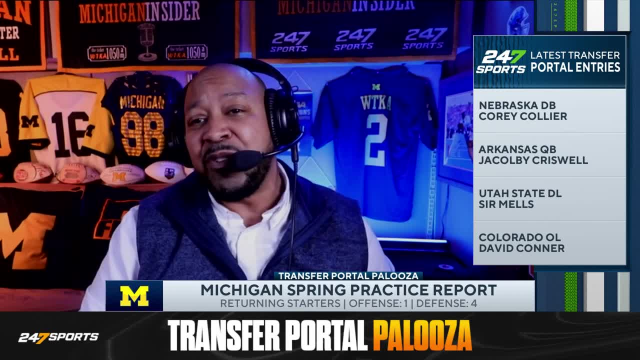 this year. The true question isn't how good they're going to be, because they're going to be first-round draft pick. The question for Michigan is going to be: how good would their depth be if they're going to be a first-round draft pick? The question for Michigan is going to be: how good would their depth be if they're going to be a 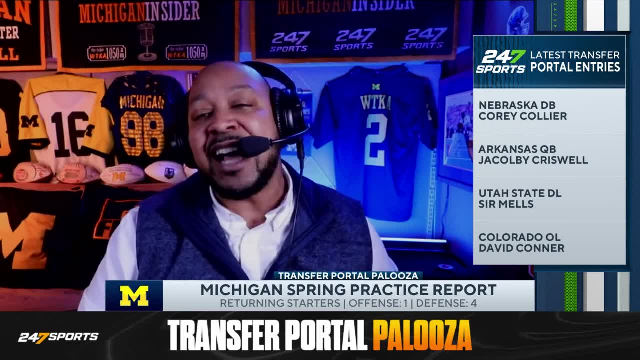 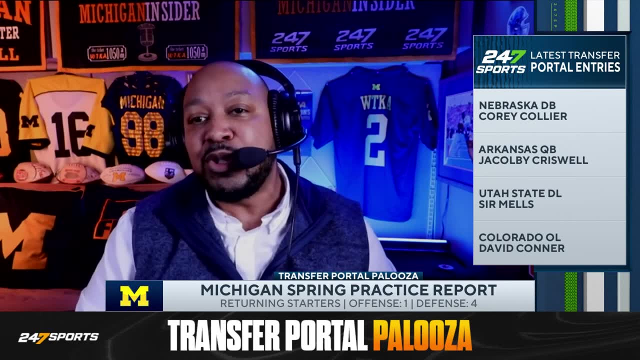 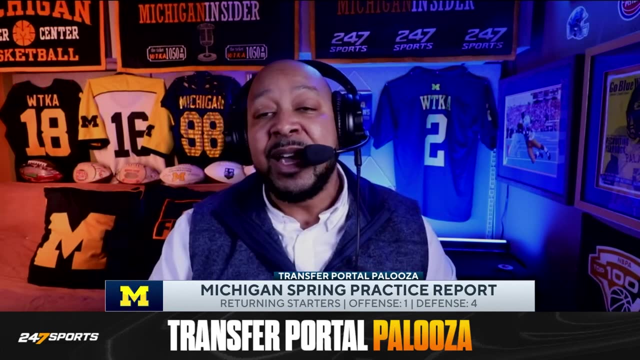 first-round draft pick was the truth. what made this team truly special? You think about they got than out of the portal. last year from from Coastal Carolina. You had Derek Moore who was the top 247 on other edge. Those are your two. 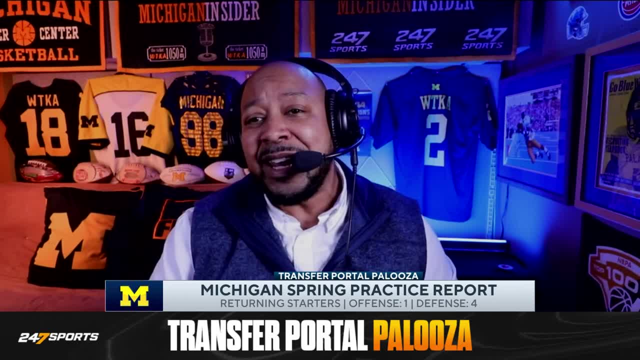 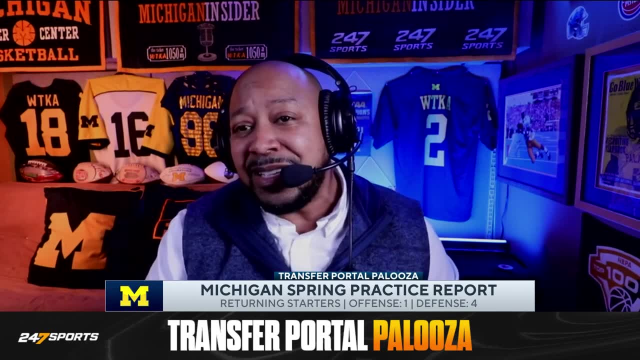 starters. this year They back-ups. last year They were back-ups to the guys in Braden McGregor and Jalen Harrell that You know. I think they were not as talented as Derek and Josiah, but they have played a lot of football at Michigan. 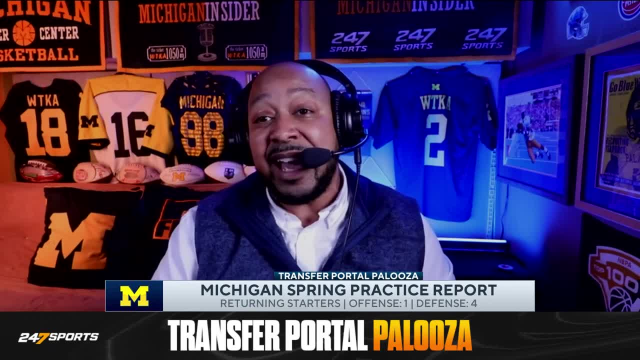 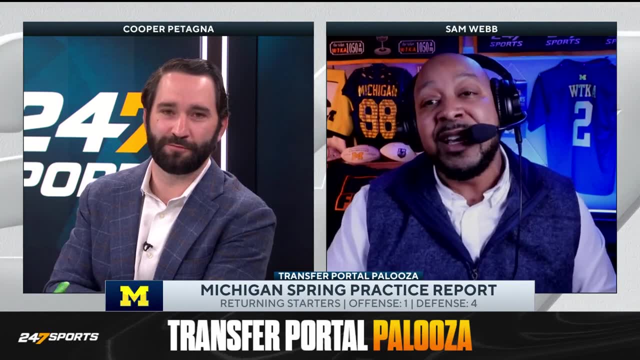 and they were able to get that rotation going. So in the fourth quarter of these games they were still beastly. The question is going to be: can they be that deep this year? Because I have no question the starting lineup is going to be as good as it was last year. 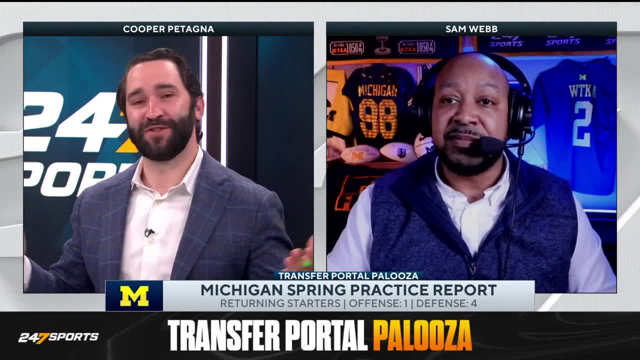 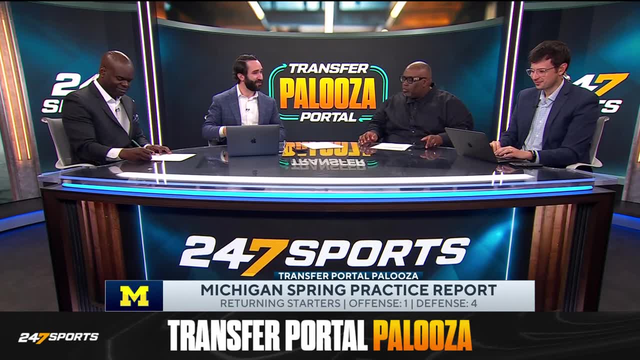 Sam Webb from Michigan Insider. appreciate you, man. Hey, Sam, great to see you, brother, as always and we'll talk soon. Appreciate it. He comes with the goods man. He's got great energy, great juice. 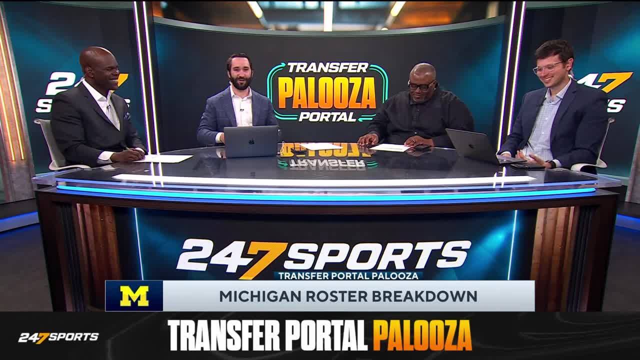 Love that guy. He's got the real recognized real report also as well that you can read. And we didn't talk about Ja'Sean Barham. That's a guy we're going to talk about in a little bit, But we're going to do the Michigan roster breakdown here a little bit. 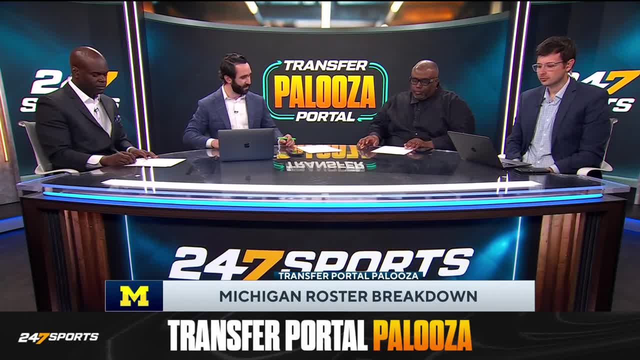 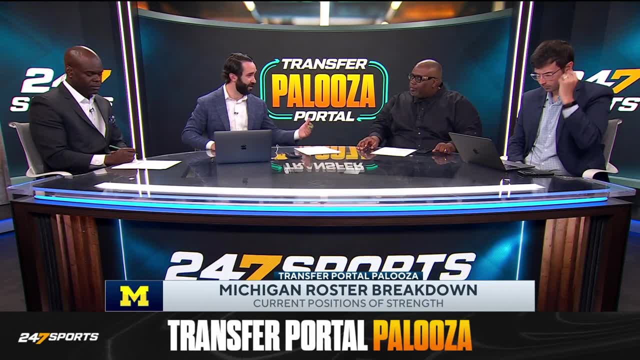 Carl, I want to start with you Positions of strength. going into the season We talked about Alabama in their secondary maybe being a position in a group that they've got to sure up, Not for Michigan. This seems to be a group that continues to get stronger and stronger every year. 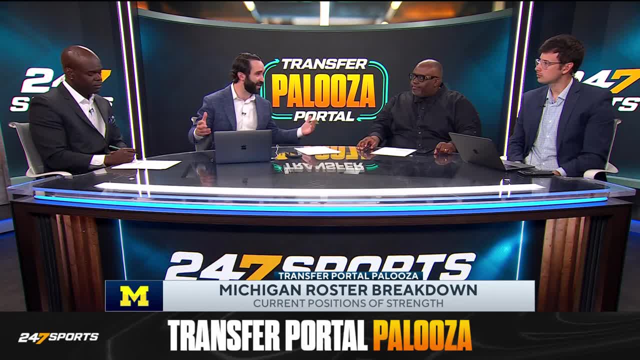 And outside of Will Johnson it's not a lot of guys that are really kind of household names coming out of high school. If they've got some talent there, what do you like about that group? Both safeties return NFL prospects, both of them mid-round type guys. 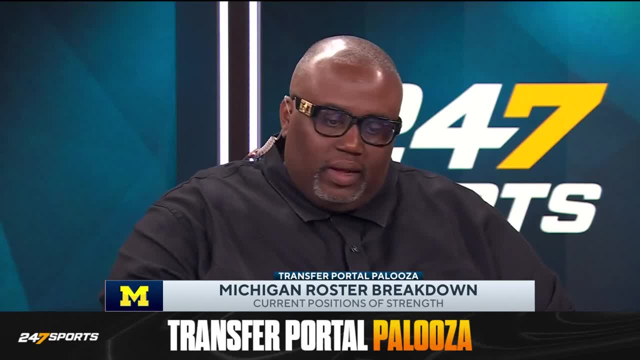 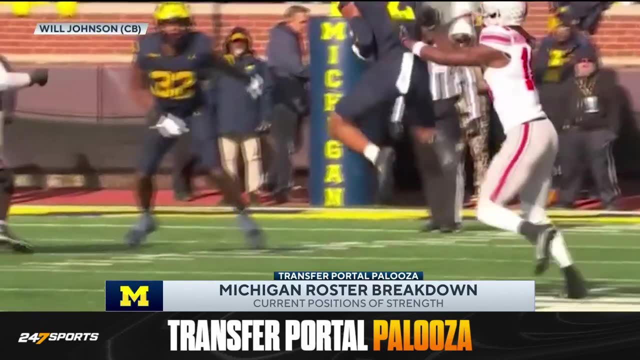 Obviously Will Johnson, who's going to be a top ten pick in next year's draft, loaded in the secondary. Great development has happened back there with the Michigan defense. They're going to come in really, really strong for the University of Michigan. 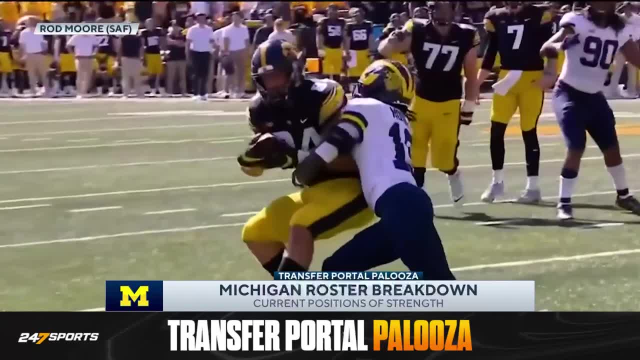 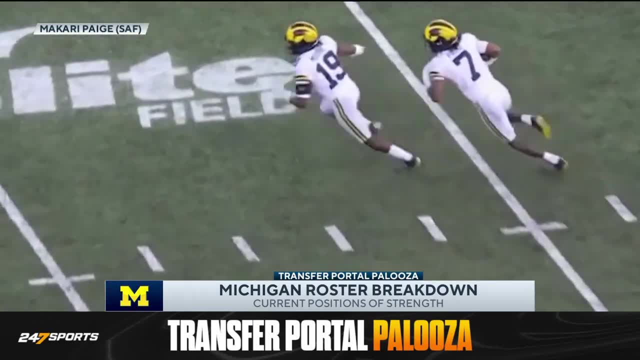 And it was good that they were able to get all of those guys to stay in the transition between Harbaugh and Sharon Moore, But they've done a really good job developing this position. Sam talked about the culture, which I think is really important when you talk about. 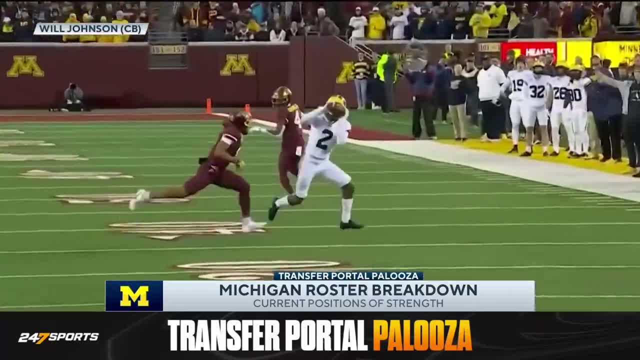 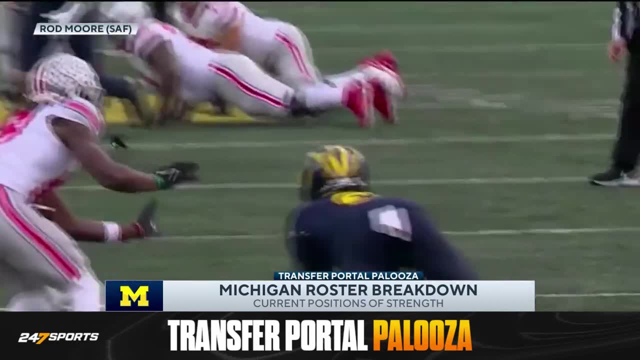 Michigan and what Jim Harbaugh was able to build there. And obviously you have the continuity in Sharon Moore. But Steve Klinkscale, he's off to the LA Chargers with his former boss, right, Not to mention the former defensive coordinator as well. 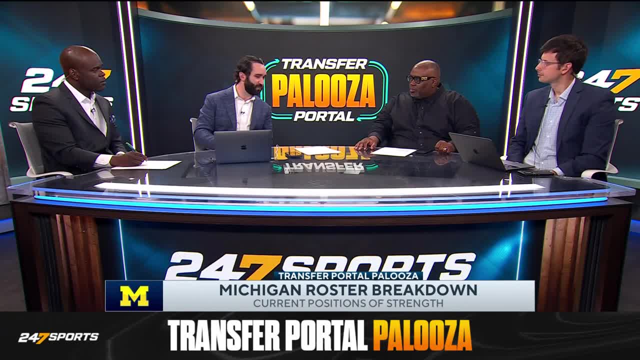 And Jesse Minter. how much does that really kind of factor in the situation when you're looking at a secondary like Michigan going from year to year. Well, the secondary being there helps you solidify the culture, No matter who the defensive coordinator is coming in after those guys. 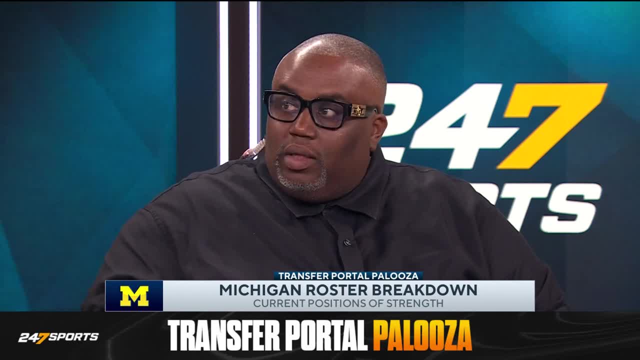 you're going to have a team that plays the same style of ball. The head coach: He's going to assess the culture and he elevated in it, he's been raised in it, And so when the new defensive guys came in, they just have to adjust to the culture. 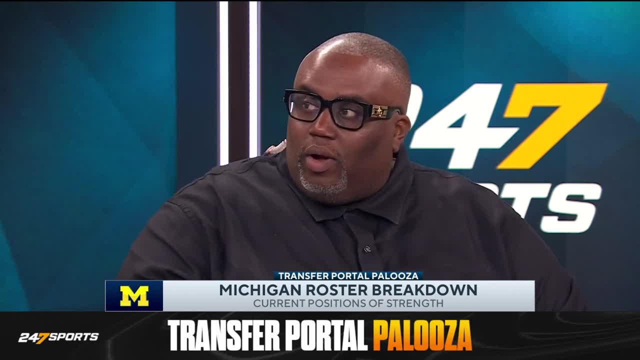 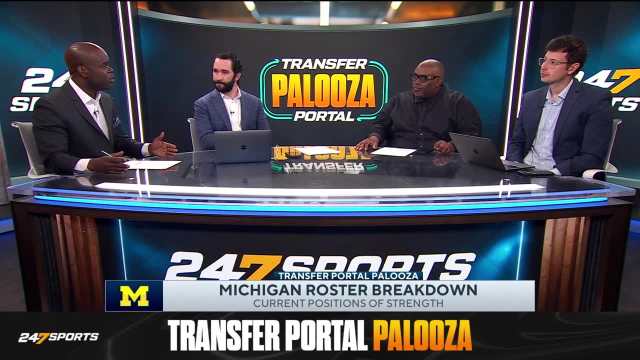 But when you have leadership on the back end like that- guys who've been in the program for a long time- it actually helps the transition of the new coaches. Well, the transition is going to be seamless. right, You got Wink Martindale coming over. 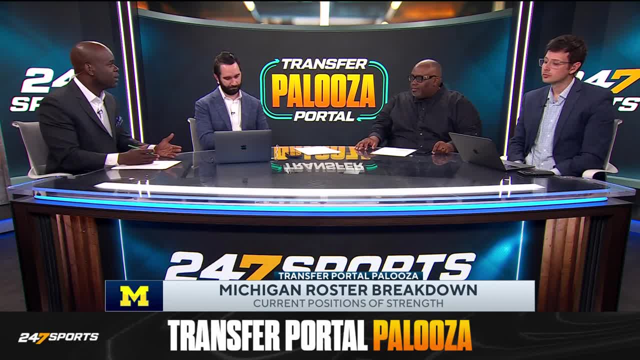 Wink Martindale is. Jesse Minter and Wink Martindale worked together in Baltimore. The new secondary coach is Lamar Morgan. Lamar Morgan, Jesse Minter and myself- we all worked at Vanderbilt, So it's going to be the same language. 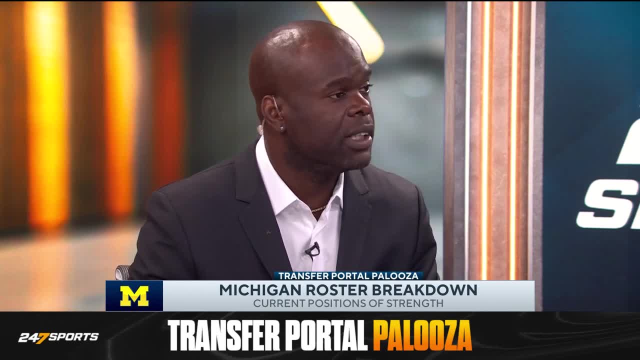 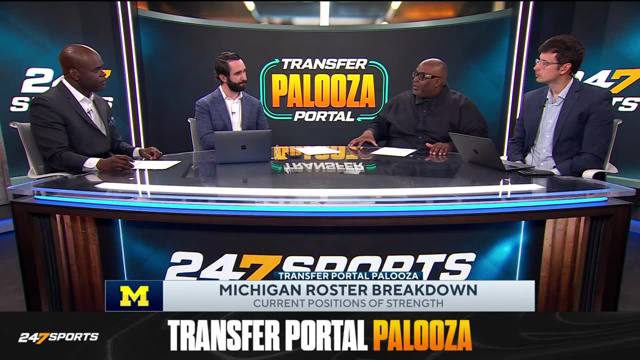 same terminology, same understanding of what you need in that defense to get them going again and contend for a national championship. And Michigan is a program that is developing guys for the National Football League. They speak an NFL language. they speak an NFL terminology. 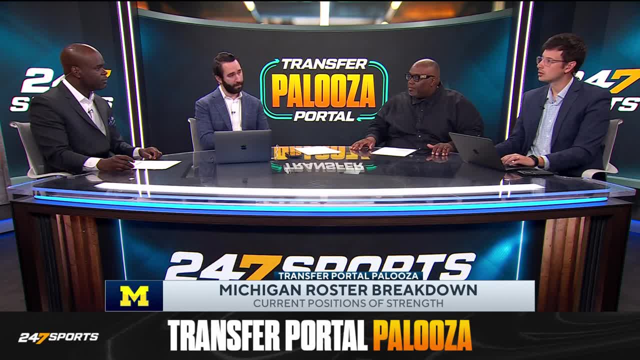 Those guys are really, really prepared to play like NFL players. And I just want to add, like I think that consistency and that development is key, because Michigan is going to have to replace Rod Moore, who's out for the season, with a torn ACL- very likely out for the season- with a torn ACL. 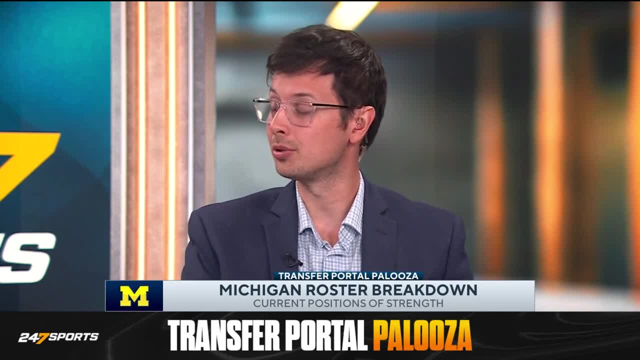 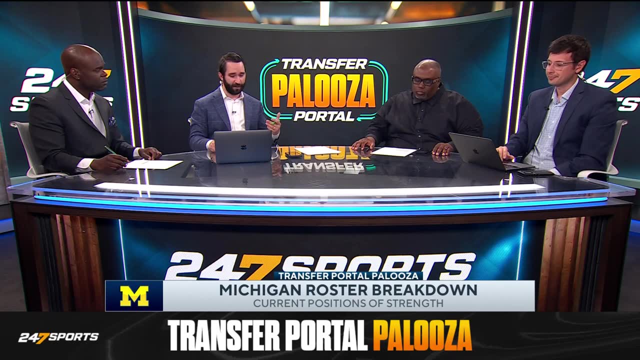 And I think their ability to develop on that back end. it's going to help Michigan kind of push through that, because they don't have brand name depth but they have depth. Chris Sam talked about that defensive line. You can't talk about that defensive line with talking about those two guys in the middle. 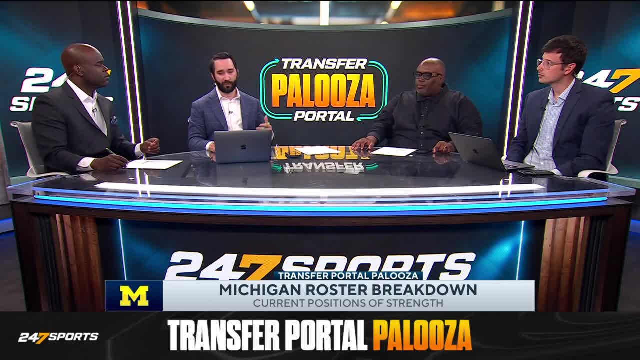 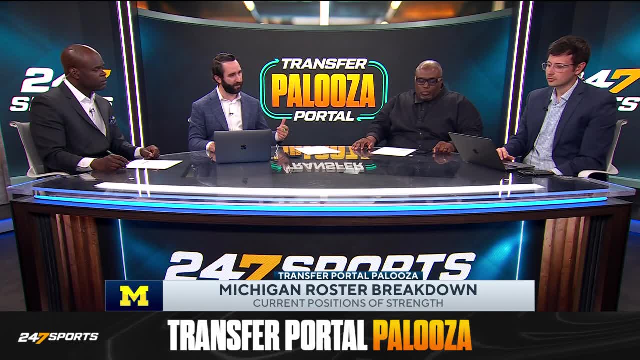 Mason Graham, Kenneth Grant- two household names now in college football, two guys that are going to hear their names pretty early in the NFL draft here pretty soon. Tell us about that defensive line group. I know Sam kind of talked about the depth. 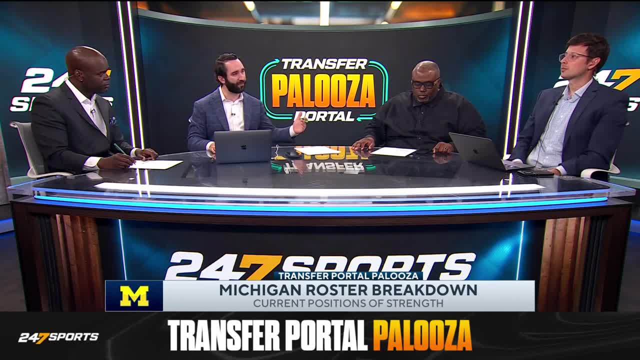 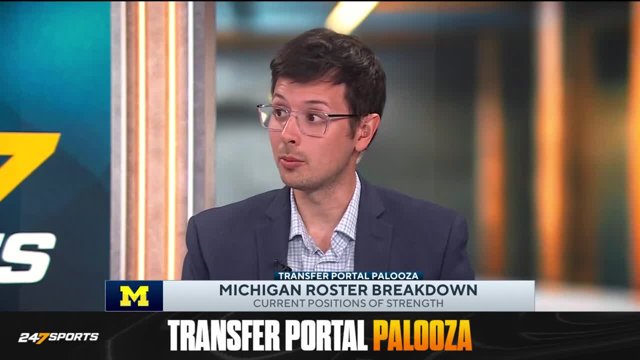 I know, Smoker, you're going to talk about that here in a minute, But what you like about that group and why that group gives Michigan a chance, Well, I mean, Sam mentioned it And you mentioned it as well- It's the best interior defensive line combo in the country between Mason Graham and Kenneth Grant. 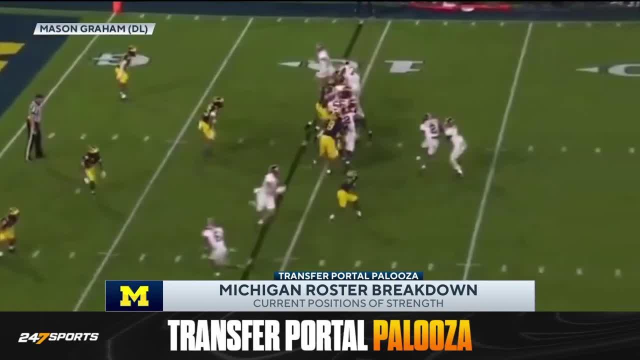 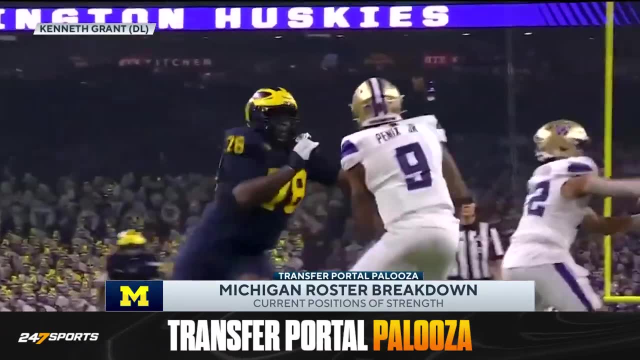 These are two defensive tackles that every single team in the country would love to have. right now- And in fact I know when Jim Harbaugh left- a lot of teams are lining up for a shot at potentially talking to them, And Michigan's done a good job retaining their roster in the wake of that. 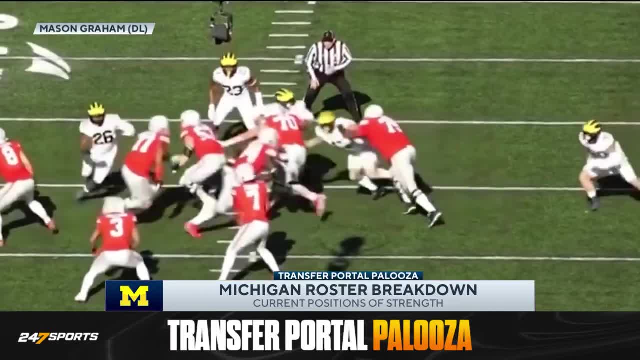 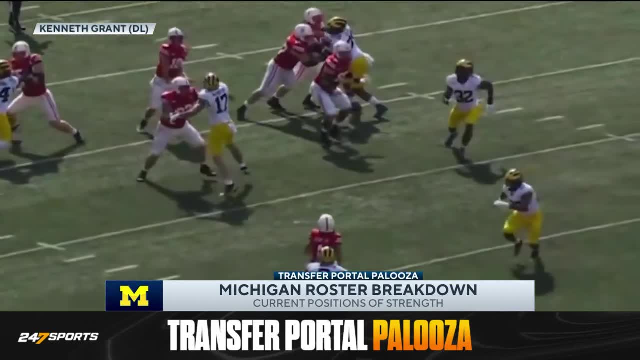 at least a lot of key players, And Kenneth Grant and Mason Graham are arguably the two most important on the roster. They are the centerpiece of that defense. They are two big guys who move in ways that big guys don't usually move, And I think they are going to continue to be a powerhouse even with Michigan losing Chris Jenkins. 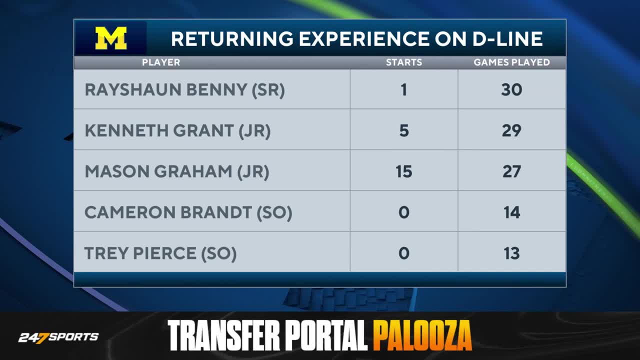 and some of that key depth that Smoker is talking about. You can build a defense around those two, And I think they're a huge reason why Michigan is projected to have a top 10 defense going into next year. We had a couple more questions for Sam, but we didn't get to get to him because, well, 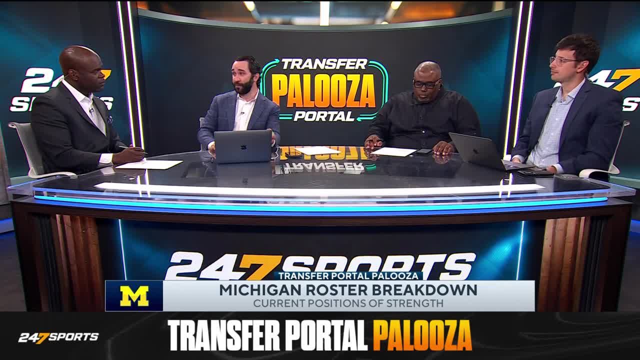 he was excited about all the topics that we were talking about, But I know he was excited about Ja'Shaun Barham, I mean certainly a guy that you're familiar with out of the DMV. You think about Josiah Stewart, Derek Moore as well. 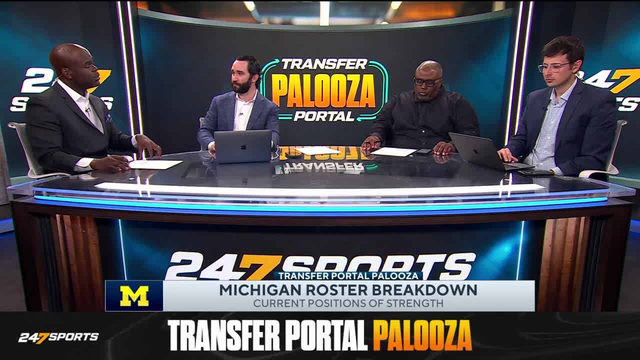 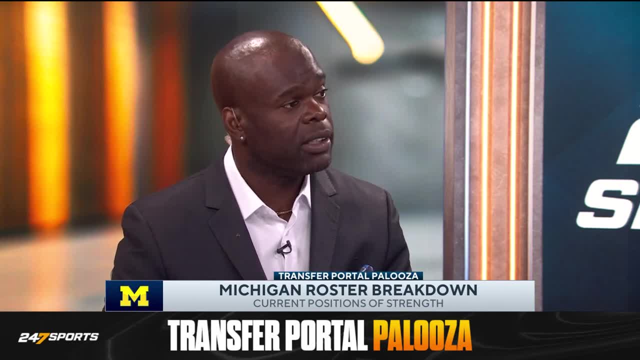 Smoke, you really really like this edge group. I love this edge group just because they can do it in a three-man rotation. In the day and age of college football, we all know it's if you have a good defensive line. 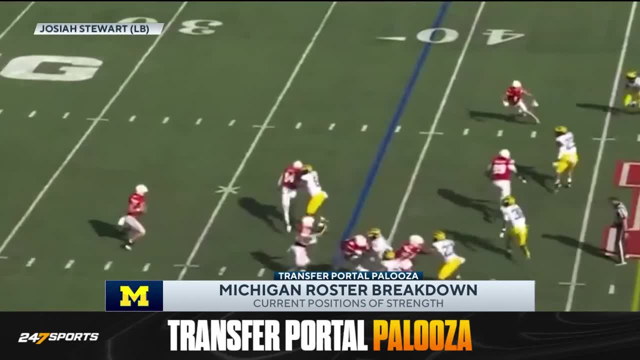 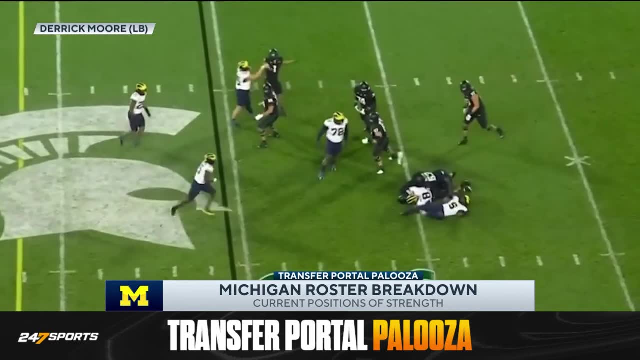 how do you nullify that? By speeding up the process. So now that you have three guys that you can rotate in there, Ja'Shaun can go on the edge and be a dominant edge rusher. He did that for Maryland when he was there. 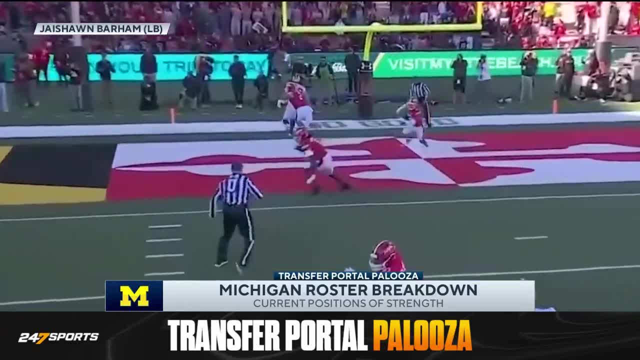 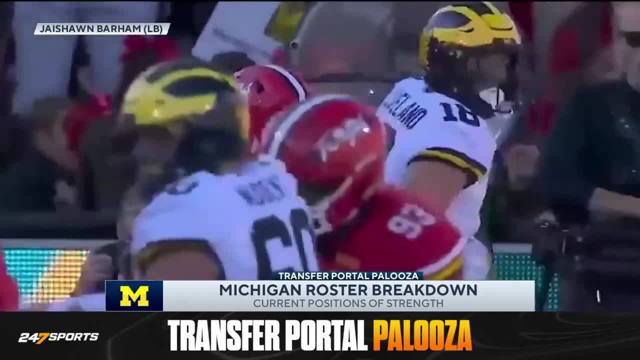 Six plus sacks. So you have two guys that are coming back that had six sacks by Stewart- 17 hurries, Six sacks, 18 hurries- And Ja'Shaun Barham can get off the edge, bend and close. 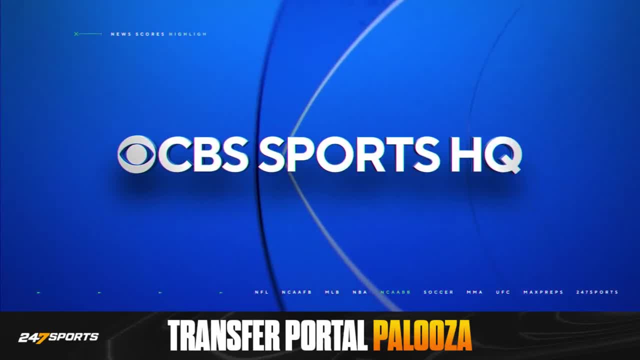 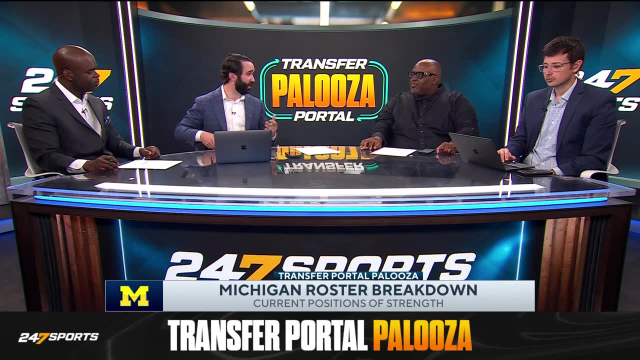 But in the age that we're in, it's all fastball. Yeah, a lot of love for him. That seems to be the name that's kind of buzzing around Michigan and Ann Arbor when you think about their spring ball. Obviously got a game coming up this weekend as well. 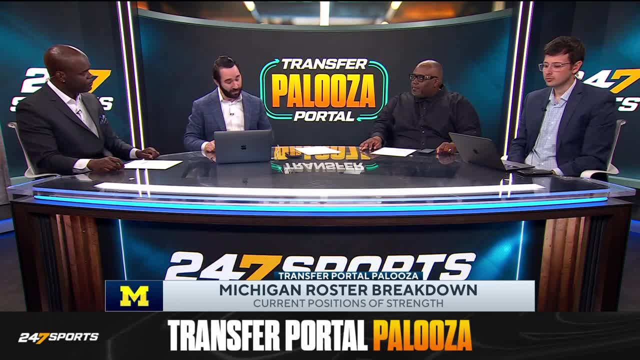 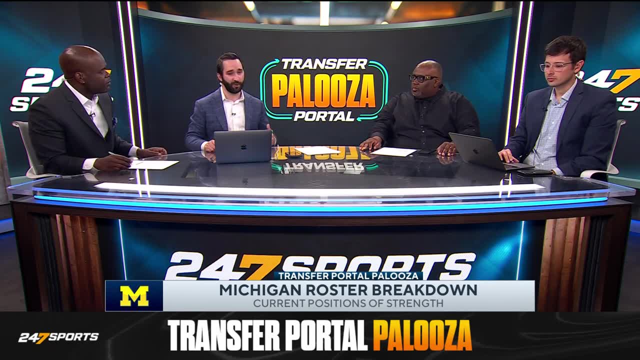 That's the name that seems to resonate with a lot of that fan base. But, Carl, on the other side, the offensive line, which has been such a strength under Jim Harbaugh, Sharone Moore over the last handful of years, You're talking about a unit that's won multiple Joe Moore awards as well. 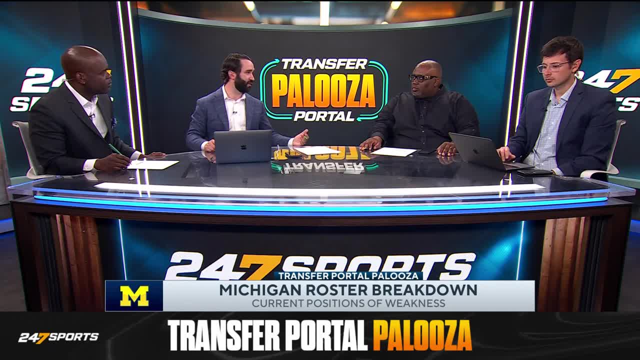 They got to replace a lot of starters, but, as Sam said, they got some experience there too, So it's not all bad news. Well, in college football, Smoke says this to me all the time: you're going to always have to replace guys. It's not like the NFL, where guys play for a decade But you lost all five offensive line starters. All of those guys are pros, run out of eligibility, left early, whatever. So when you lose five guys, there's going to be a change. 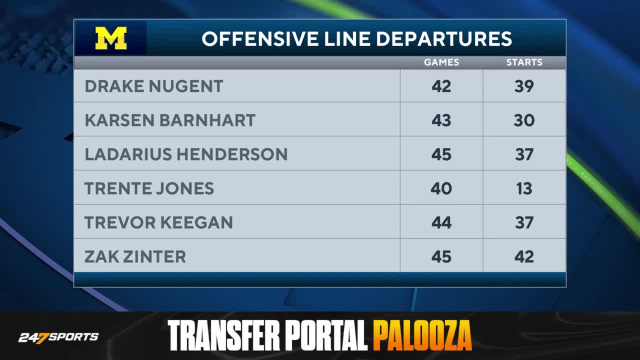 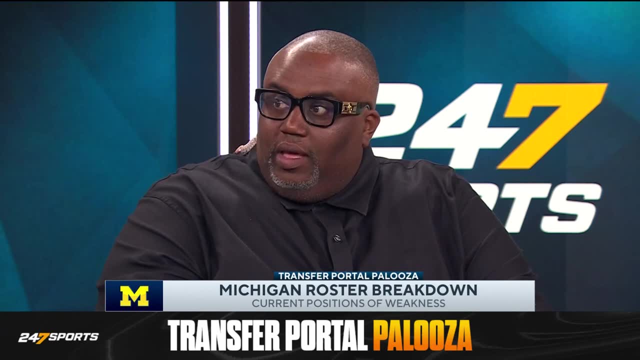 If anybody, though, was built to be able to handle this, it's Sharone Moore and the University of Michigan, So you're more believing in him than believing what you've seen, because you haven't seen these guys produce yet. But when you lose five guys- and you also lost a quarterback- this is tough to replace five. 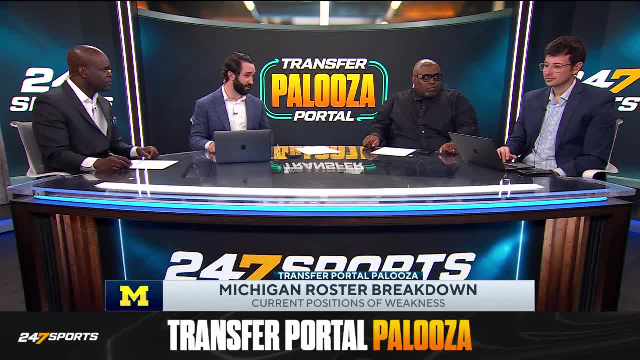 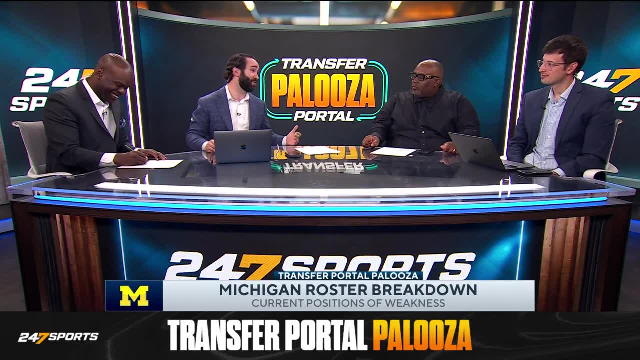 offensive line starters. Chris, you famously told me this morning looking at the rundown at the receiver position that Michigan they got nothing And that's no disrespect. I thought of some people around the program that told me the same thing yesterday, right. 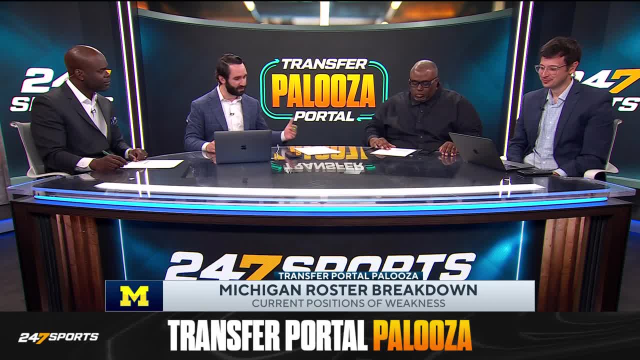 So they got some work to do at the receiver position. What's your feel on that group moving forward? They're going to have to add multiple players. They're going to have to add multiple players in the portal if they want to be successful next season at receiver. 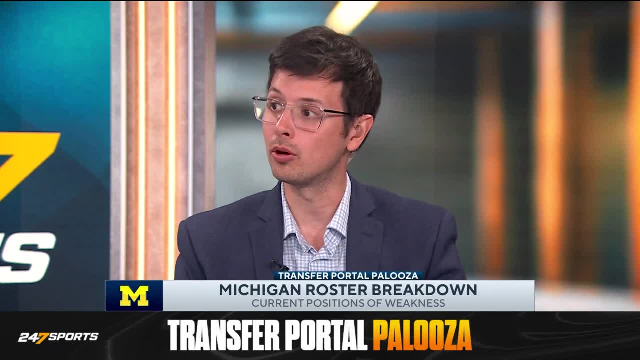 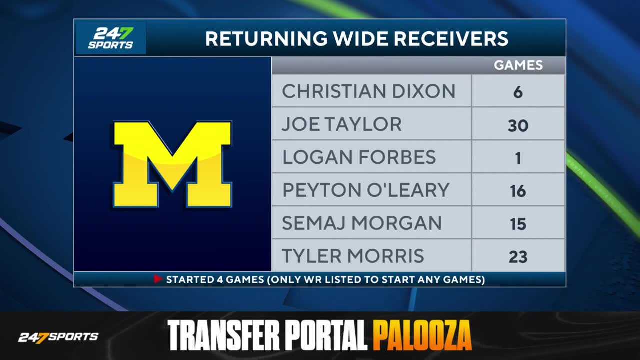 And Alex Orji is going to take a lot of that load. Obviously, Michigan is going to be a more run-focused offense this year, just due to the strength of their roster, But they don't return a single receiver who had more than 250 yards last season. 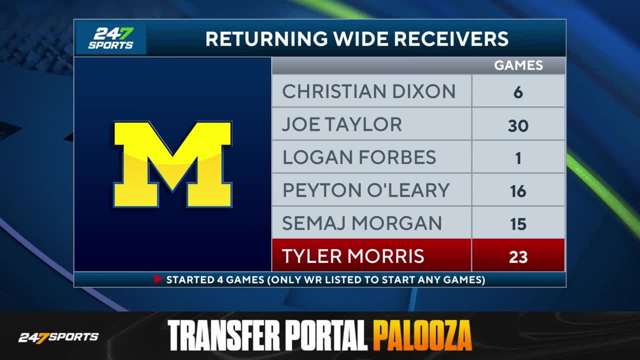 And you can count on Colston Loveland, who's going to be arguably the top tight end in college football next year. But you have to have some guys on the outside that can make plays to make life easier for a potentially inexperienced and young quarterback. 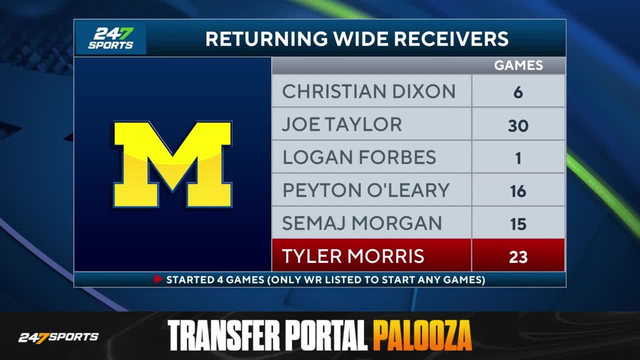 And I think that's going to be a focus for Michigan. in the portal They're going to look to get one big outside X receiver. I think they could use some more speed as well. This is something Michigan knows it needs to address and will address aggressively. 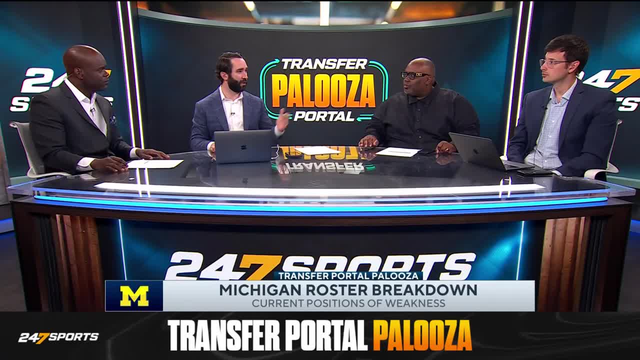 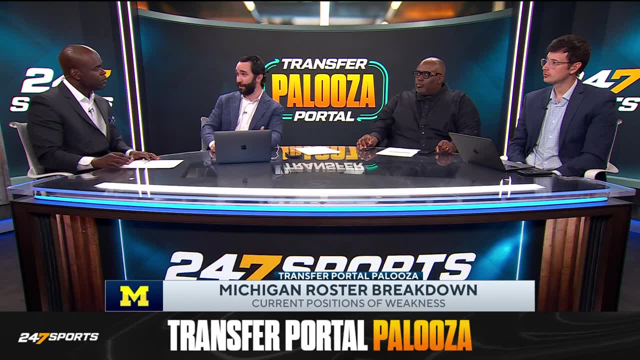 Could be some multiple guys that they take Just a couple of warm bodies as well, I think. big expectations for Tyler Morris. We kind of saw some things from him in the college football playoff smoke. I got to admit this one kind of made some people scratch their head a little bit when 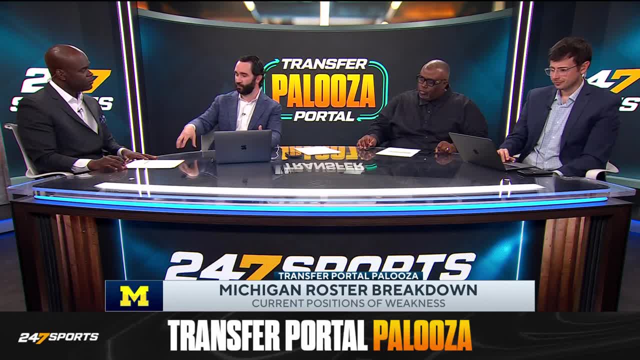 we saw this on the rundown- But that defensive line group, the same one we talked about as a strength- Sam brought up the point about the depth. I think that's something that we need to keep an eye on going forward. And don't get me wrong, 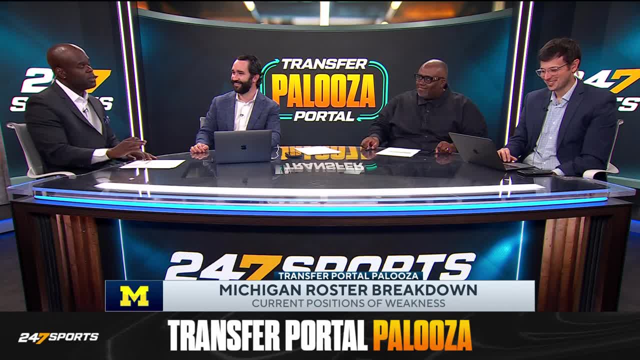 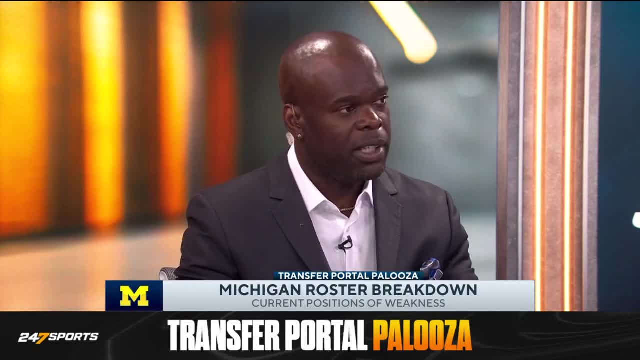 I make a lot of people scratch their head, Just because I don't really view things in the same lens that everybody else does And I'm looking at this in the total roster construction and how they play football at Michigan At Michigan, the reason why their defensive line was so tough last year- they wore you. 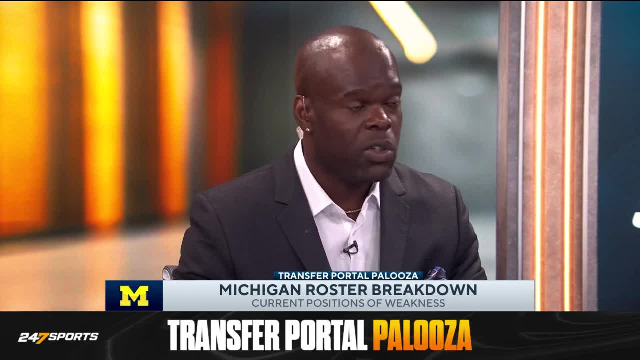 down. They rolled eight through there And if you can roll eight guys through there, you're going to be ready in the fourth quarter and getting ready to play the way that they want to play. How did Michigan beat a lot of team last year? At one point they ran the ball 20 plus times against Penn State And wore them down. How did they beat Alabama In that overtime? Bama did not want it anymore because their guys up front were ready to go. Now, when you look at it, the two guys top dogs. 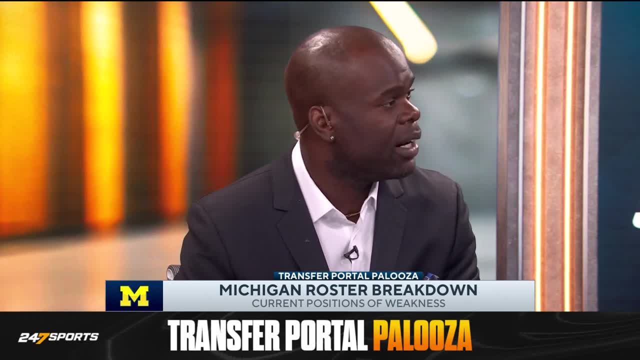 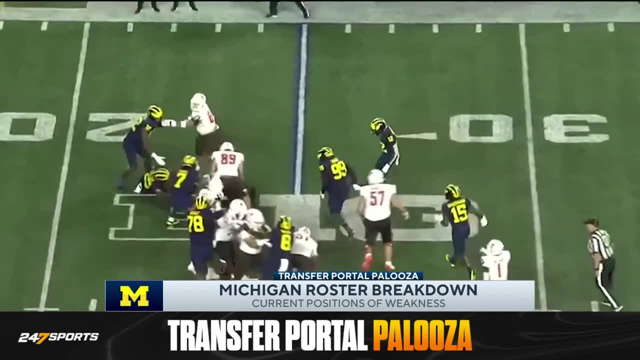 They can play. But how do you nullify that? Speed them up, Get them tired, Get them off the field. And now the others got to come in and play and make plays. And if you can keep the others in and the two guys can't get back in, now you have an. 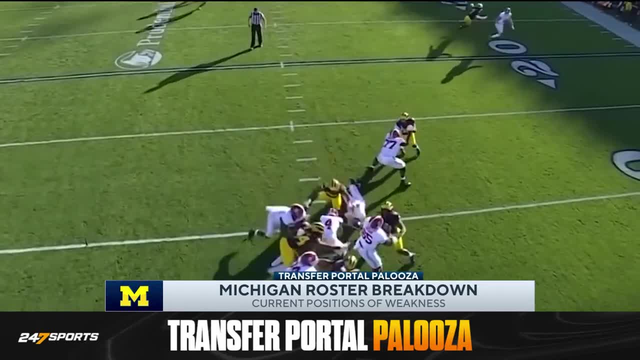 advantage. So it's really for me it's more depth than the top end guys. Top end you're really good, But in college football you've got to have a middle of the group because you've got to be really good. 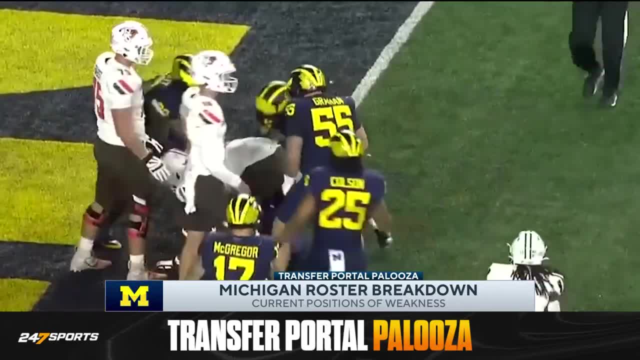 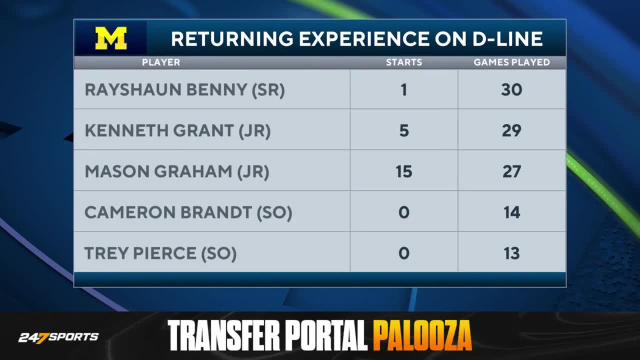 And your bottom end has got to push that middle of the group And Smoke. what's made a lot of those championship teams special over the last ten years has been depth. It's when you played Alabama and Georgia and Michigan and Ohio State Guys went down. they replaced them with another guy. 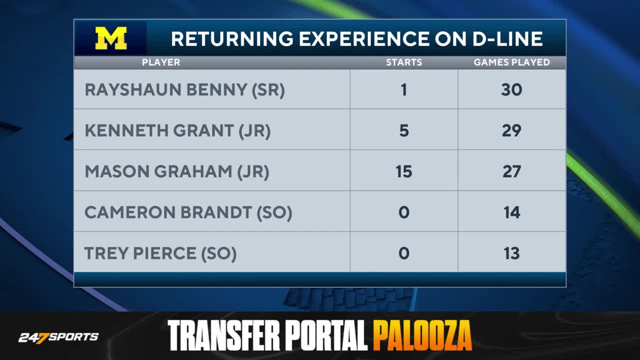 Guy go down, they replace him with another guy. This guy subs out, you replace him with another guy, And so that's kind of what the transfer pool has done. It's killed depth in a lot of situations. Chris, a lot has been said about Michigan.